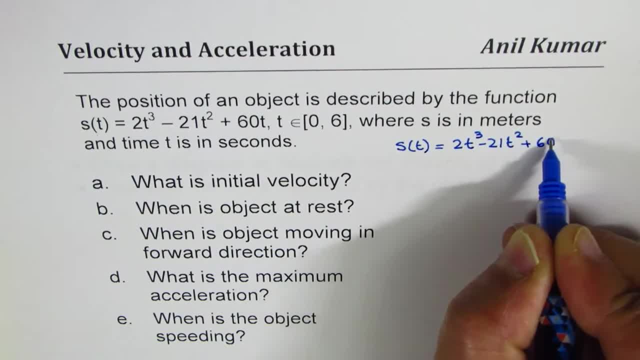 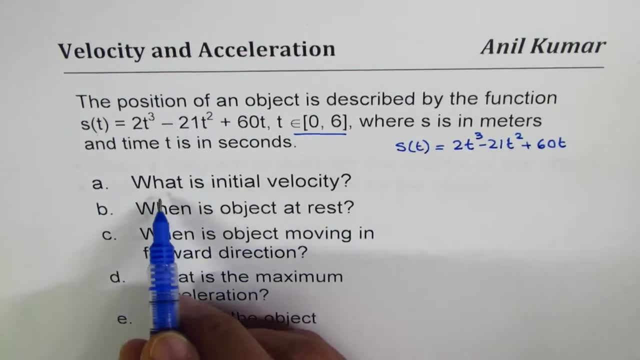 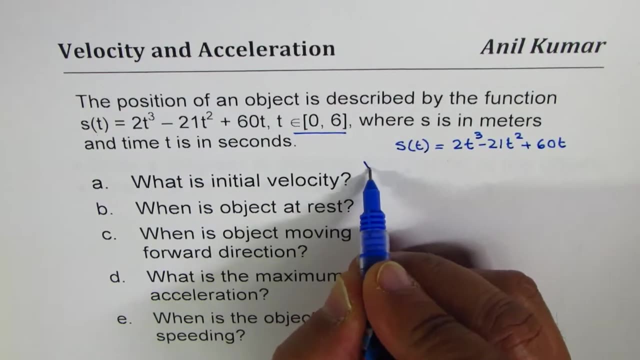 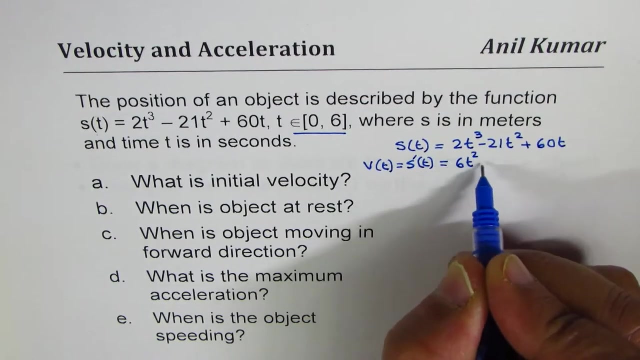 plus 60t. remember, the interval is from 0 to 6. what is initial velocity? first derivative of displacement is velocity. so velocity is equal to the derivative of displacement or position with respect to time. so you get 3 times 2: 6, we get 6t square minus 2 times 21, which is 42t, and here we get plus 60, right. 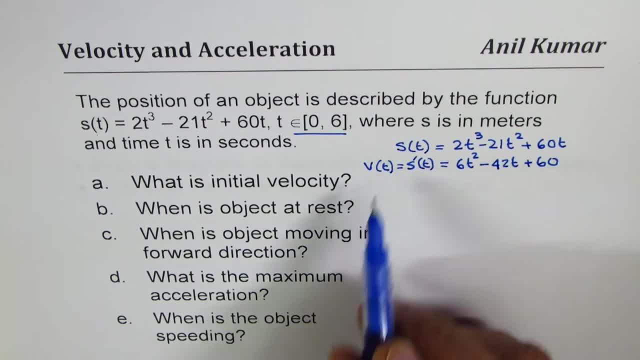 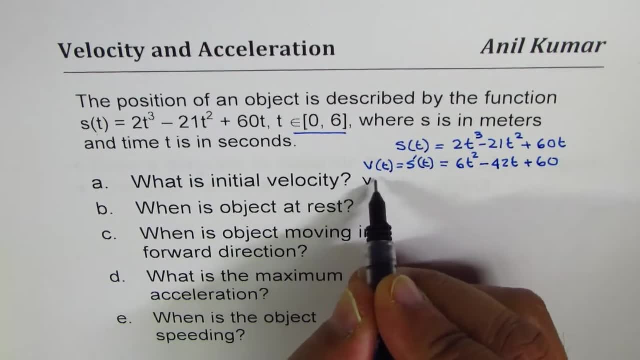 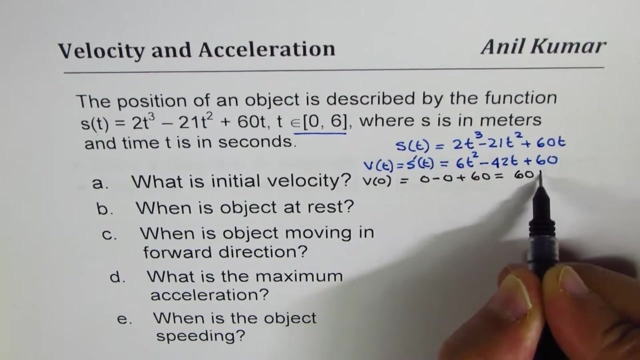 so that becomes an expression for velocity. what is initial velocity? that means t equals to 0, right? so initial velocity is v of 0 equals to. if I substitute 0 here, I get 0 minus 0 plus 60, right? so I get 0 minus 0 plus 60, which is 60 meters per second. always include units. 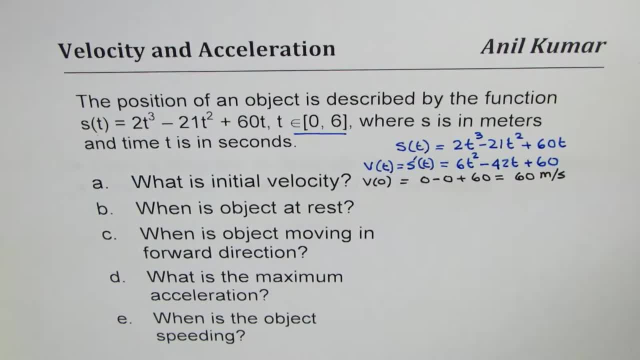 in your answers whenever you're working with velocity and acceleration. the next question here is: when is object speeding? and in continuation we'll look into the distance traveled by the object speeding and acceleration. the next question here is: when is object speeding and acceleration? the next question here is: when is object? 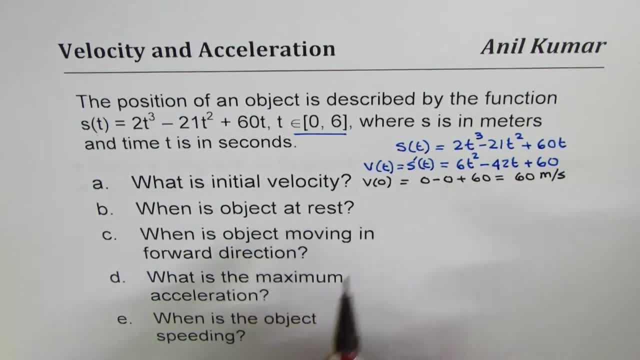 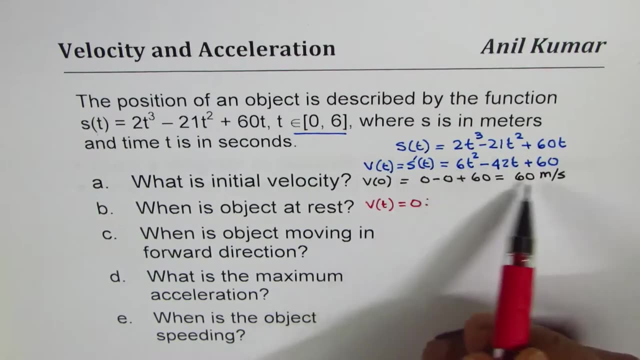 at rest. object at rest means that the velocity is equal to 0. right, then, the object is at rest. we have this expression for velocity: 60 square minus 42, t plus 60. if you equate this to 0, we will. we can find t right. so let's rewrite this and while writing, I can. 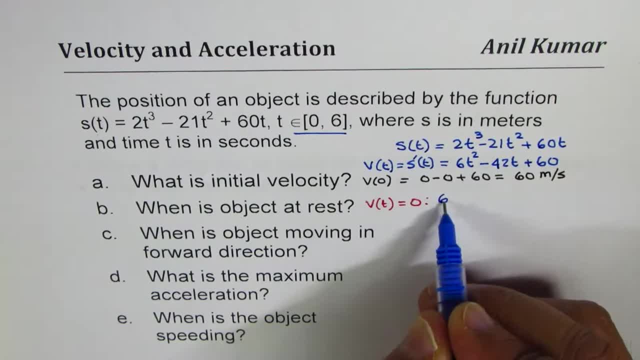 take 6 common with right. so if I take 6 common, I'm left with t square minus 6 times 7 is 42 and 10. this should be equal to 0, for velocity being 0. that is when the object is at rest, right. so this: 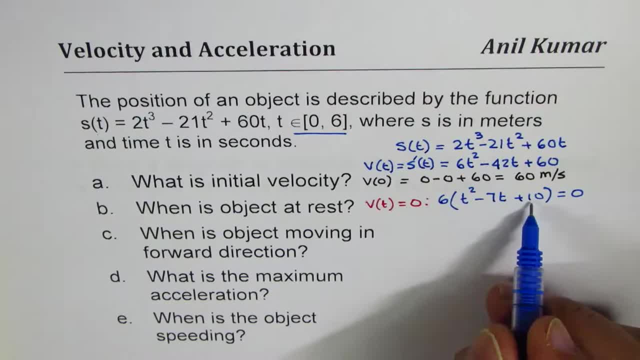 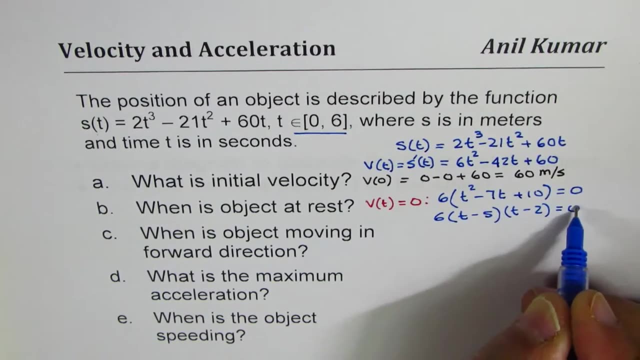 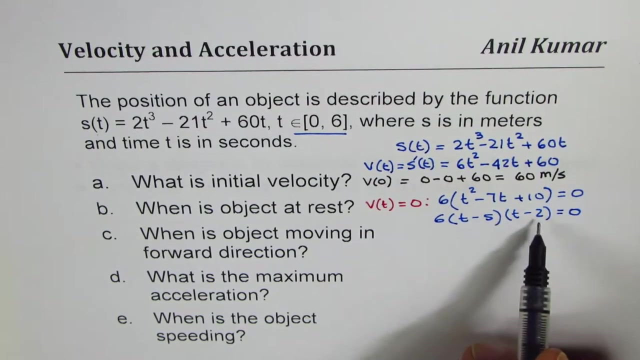 could be written as now: product: we want 10 sum as minus 7, so the two numbers are minus 5 and minus 2, so we can write this as t minus 5 times t minus 2 equal to 0. now when is this expression 0? it is 0, at t equals to 5 and at t equals to 2, right? 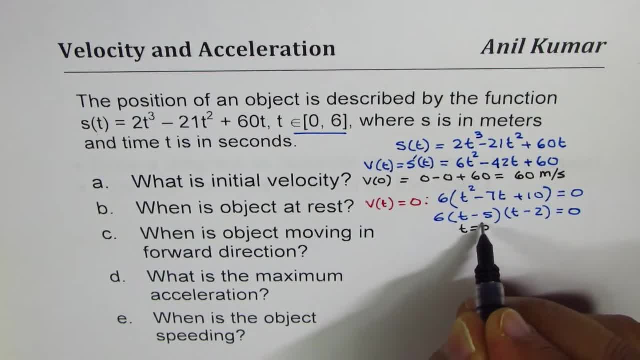 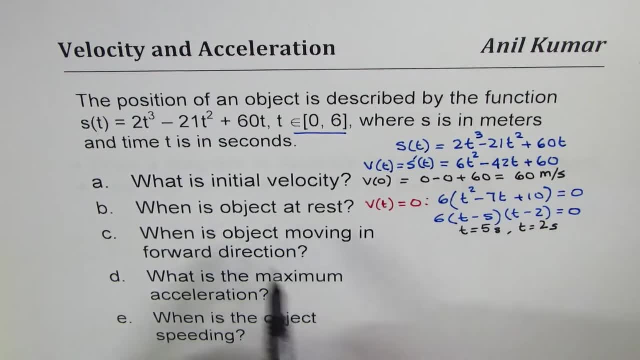 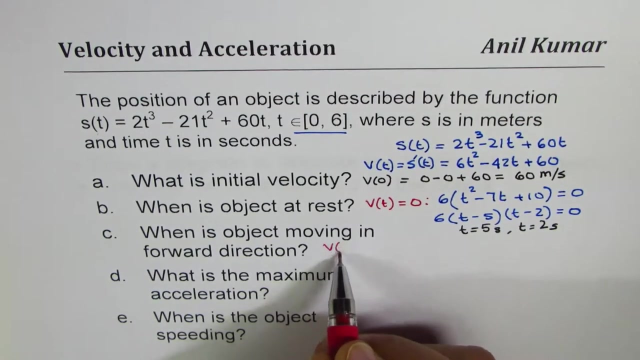 so those are the two answers: t equals to 5, the units are seconds and at t equals to 2 seconds. at that time the object is at rest. part C: when is object moving in forward direction? forward direction really means that the velocity is positive. right, so that means velocity is greater than 0. 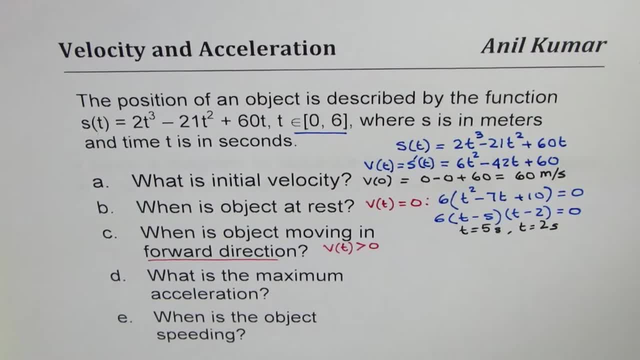 that means forward direction, right, so let's figure it out now. one is: we have this expression for velocity in factored form, which is a better expression to use now, so let me rewrite this. we say velocity could be written as 6 times t minus 5. 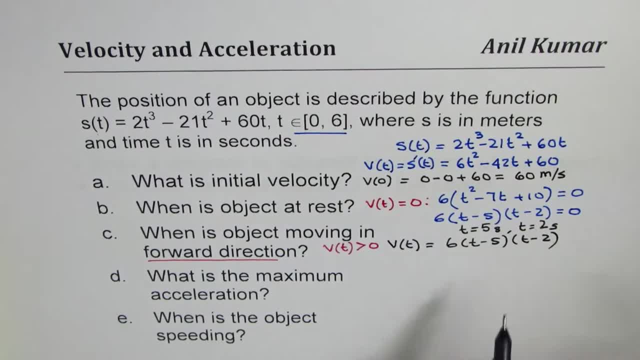 times t minus 2, right, you can solve this inequality for greater than 0 to know when the object is moving in forward direction or the alternate is. you could sketch this parabola right, which I prefer to do less calculations right, and I always like to solve questions in minimum space. so what? 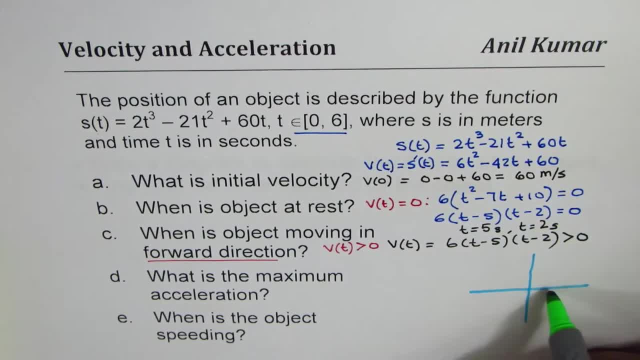 we can do here is: I'm more interested in these x-intercepts and not really the value of the graph, so I'll just draw a parabola kind of like this: right, okay, I should actually stop at 6. the two zeros we are talking about are at 2 and at 5. 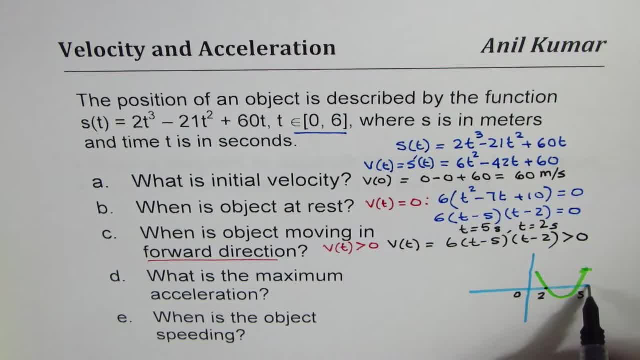 correct object starts at 0, ends at 6, so that is the duration which we are interested in now when the question is: when is object moving in forward direction? from this diagram it is very clear that velocity, this is velocity with respect to time. here we have time. it is positive in. 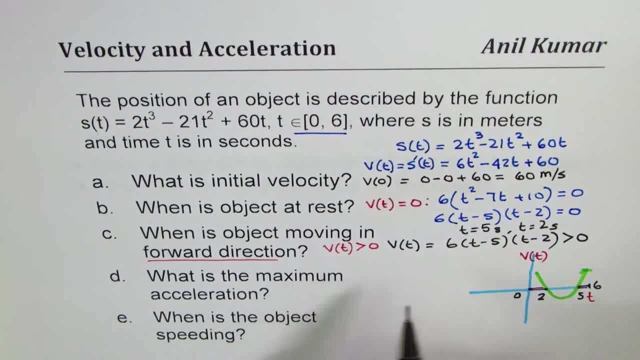 this position correct? so the answer here is: it is moving in forward direction in the duration of time. so it is the acceleration from 0 to 2, and or you can write union right- 5 to 6. this is the portion where velocity is positive. right, this was positive. the next part is: what is the maximum acceleration? now, to find acceleration, we have to find derivative of velocity, since acceleration, you know, is equal to derivative of velocity. 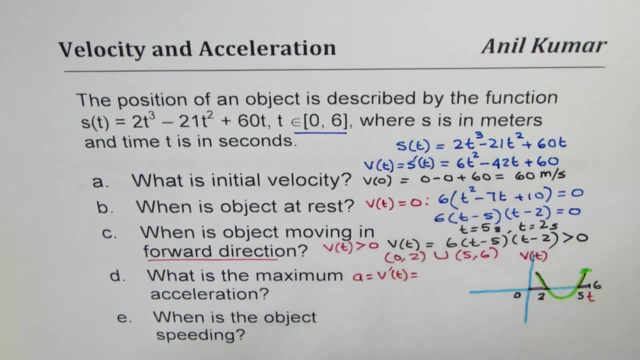 So for derivative I will prefer to use the standard form. right Now we can find derivative: 6 t square gives us 12 t minus 42, minus 42. So that becomes the expression for acceleration. We want to know what is the maximum acceleration. Now this is a straight line, correct At t. 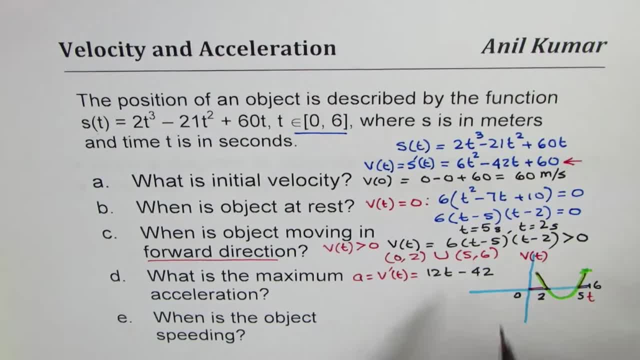 equals to 0, at t equals to 0,. it has a boundary condition. the boundary condition is from 0 to 6, right. 0 to 6, correct. Since there is no turning points, just a straight line. what we can do is we can find value of acceleration at 0 and at 6, right? So 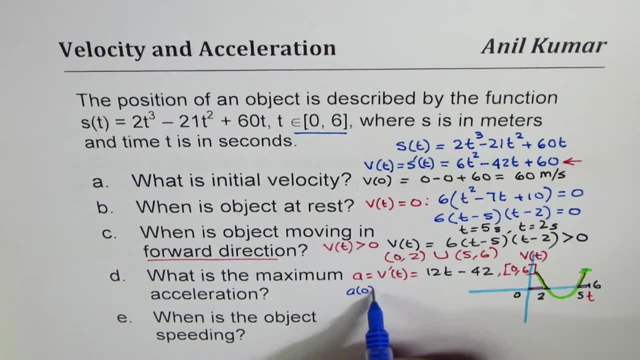 we have acceleration at 0, will be minus 42, and acceleration at t is 8, we have AO, capital factor k, So we need to have Moripi plains as m plus stronger than 0. Similarly, then T is 23.. We try to. 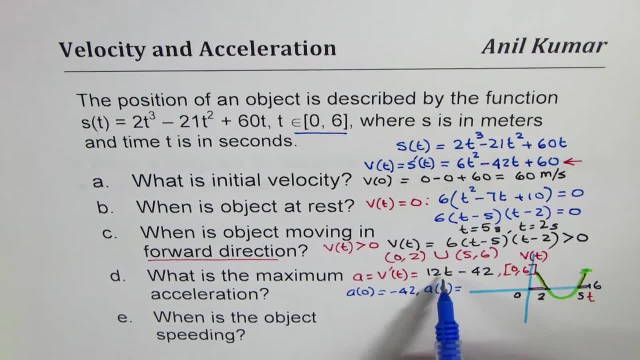 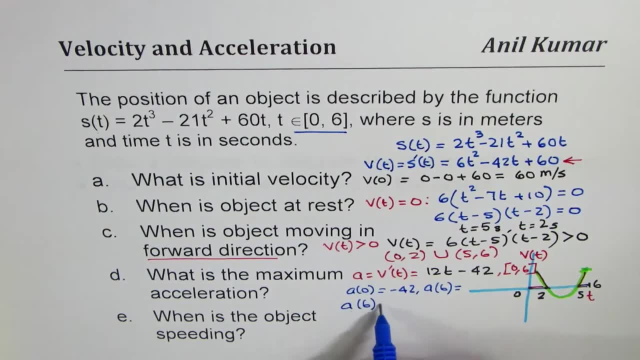 at 6 will be: we can do 6 times 12. okay, so at 6 it will be. we can do here right. acceleration at 6 is equals to 12 times 6, which is 72 minus 42, so 72 minus 42. 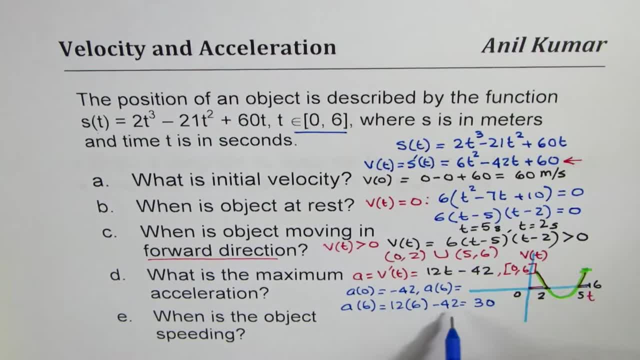 gives us 30, correct 72 minus 42 gives us 30. and when is it 0? well, let's find that also okay. so let's calculate that also. we may need it in part. e when is the object speeding? so we might need it soon, so we'll find. when is acceleration equal? 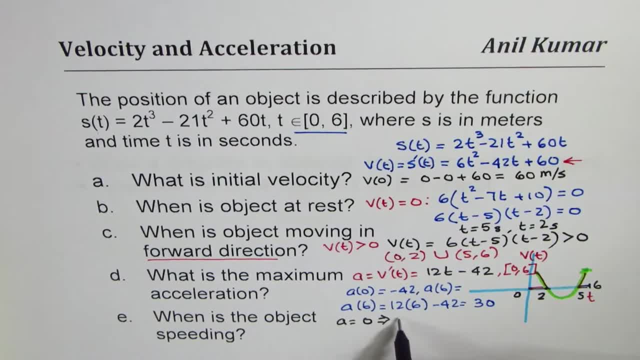 to 0, that is to say 12 T minus 42 equals to 0, and that gives us T equals to 42 divided by 12, right? so 42 divided by 12, 36 plus 6 is 42, so we get 3.5. okay, so at time, 3.5 it. 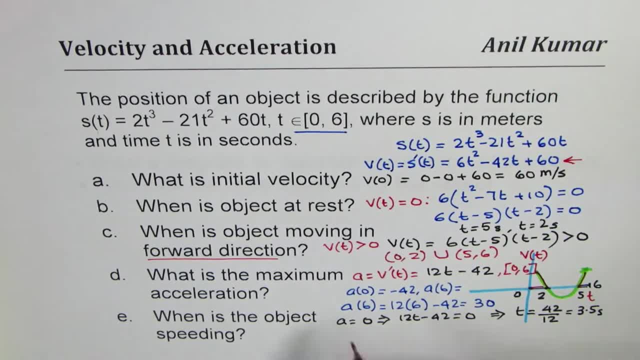 is 0, so we can actually sketch the straight line 12 T minus 42, kind of. let's start from here saying this is minus 42, going through 3.5 in the middle right. let's say this: so that becomes the acceleration part, and clearly we see that acceleration is maximum at its limit. 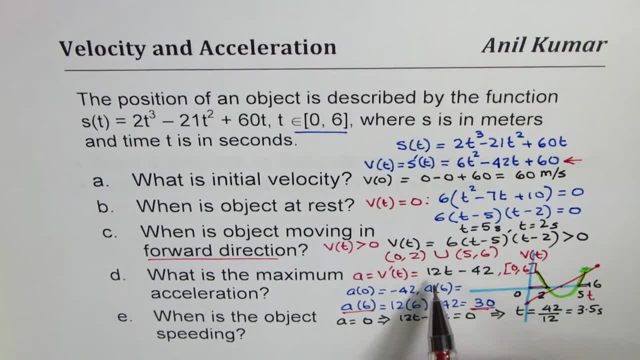 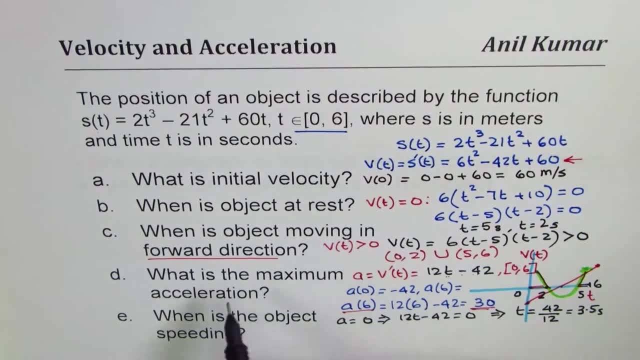 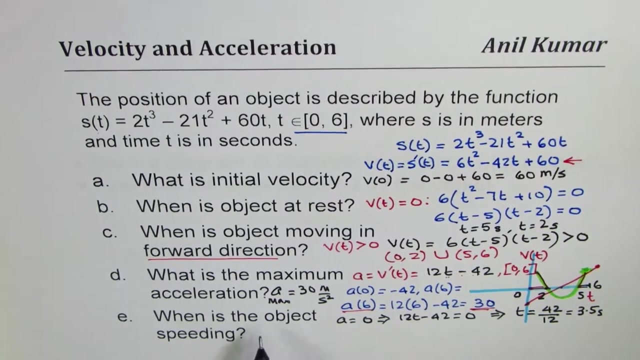 which is 30, right, the highest value. so this function, 12 T minus 42, is always increasing, correct? so let me write down one answer here: what is the maximum acceleration? so maximum acceleration is equal to 30 meters per second square. perfect, now, when is this? 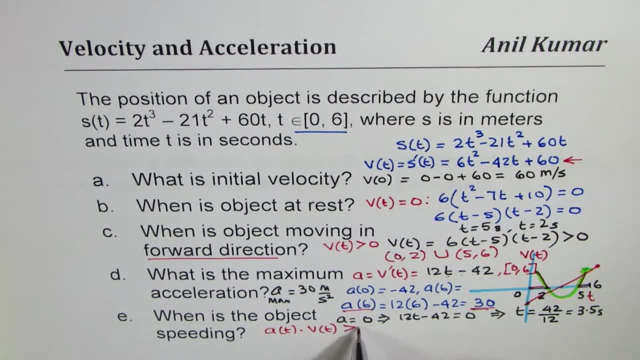 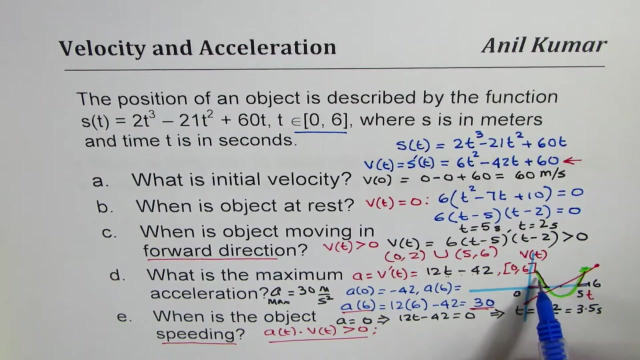 Jerry, are you right? plus 1, 0, 1 A, 0, 0, both positive, correct. now from this graph, what do you observe? which interval do you think they both have the same sign. can you help me find this answer? okay, as you can see, in the interval 0 to 2, velocity is positive, acceleration is. 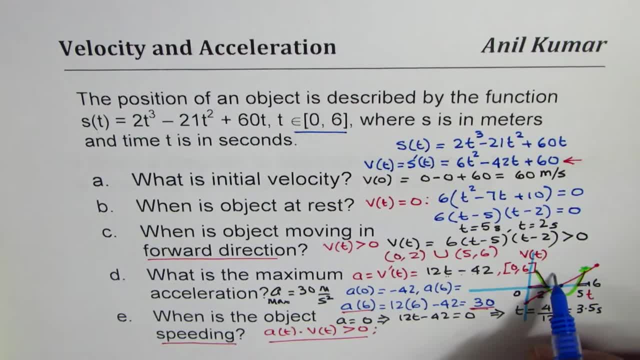 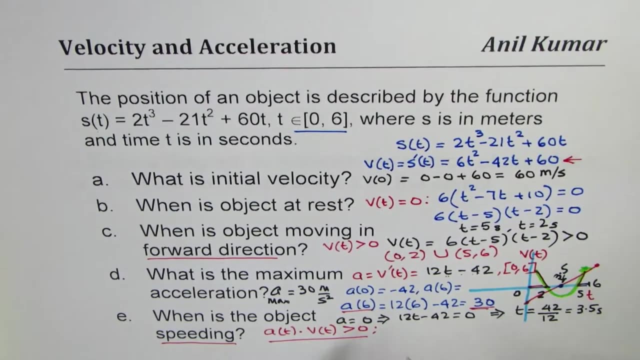 negative, but from 2 to 3.5. this point is 3.5. let me write here in a different ink so that 3.5, which is this point, right from 2 to 3.5. both are negative. so one of the interval is: from 2 to 3.5. right, both are negative and then both. 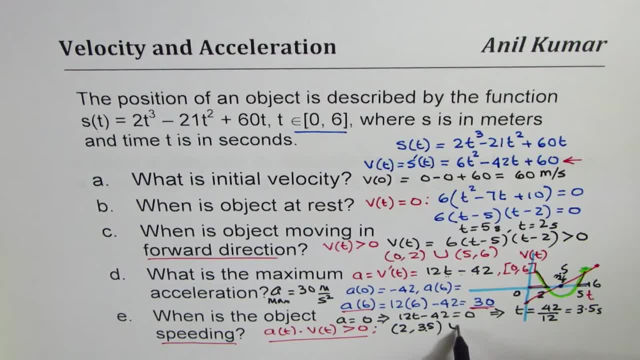 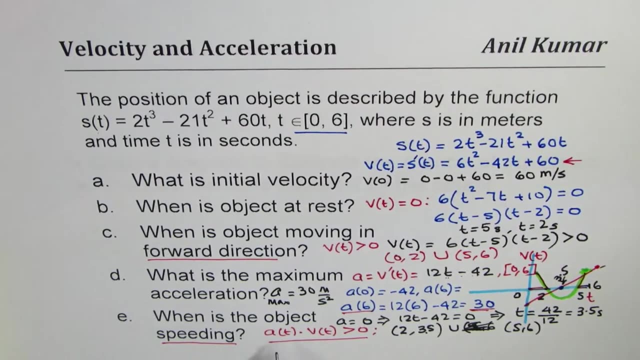 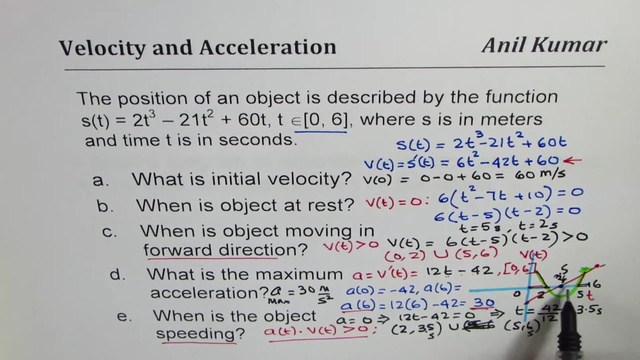 are positive after five. so the union from five to six. right from I mean five to six, five to six, ok, five to six. so from this graph it is very clear that they are speeding in the interval from two to 3.5 seconds and from five to six seconds. correct both. 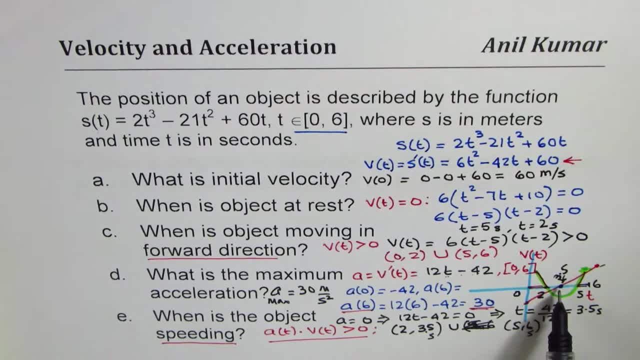 are negative in the into well, to two to three point five, and both are positive in the interval 5 to 6, correct? So these are the two intervals where they are speeding, correct? So I hope that is absolutely clear. So with this we have answered these five questions. And now 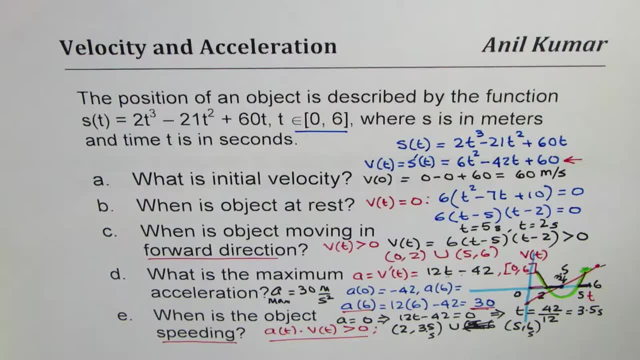 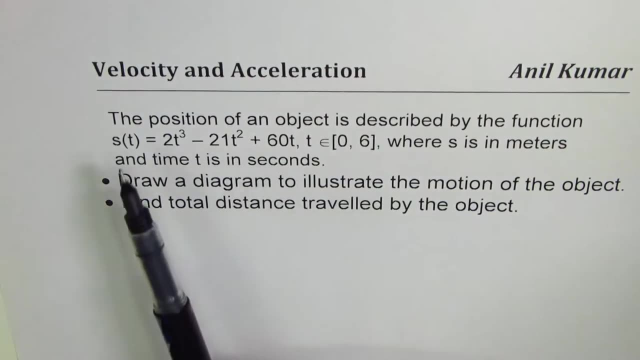 I will move on and we will take up another important aspect, which is displacement and distance. So we will discuss both in the next page, right? So here we have the same question with the additional two parts. It says the position of an object is described by the 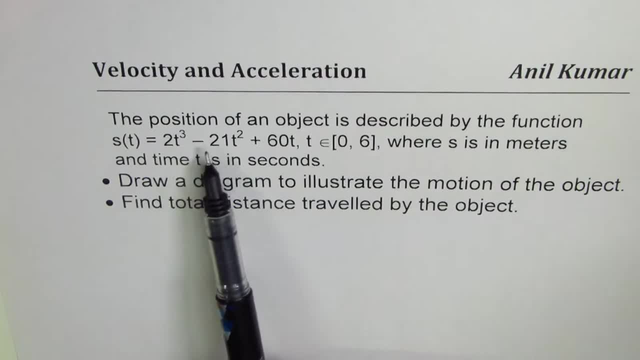 function s of t equals to 2t cube minus 21t square plus 60t. t belongs to the interval 0 to 6, both included where s is in meters and t time is in seconds. Draw a diagram to illustrate the. 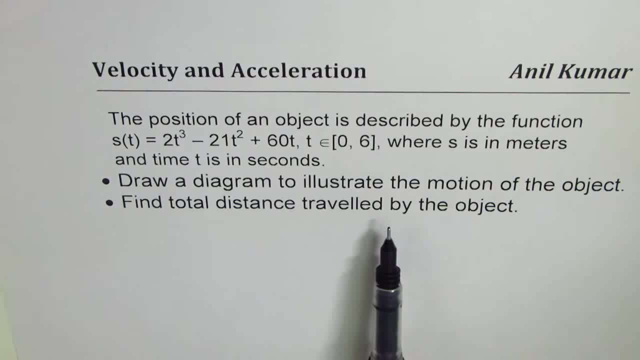 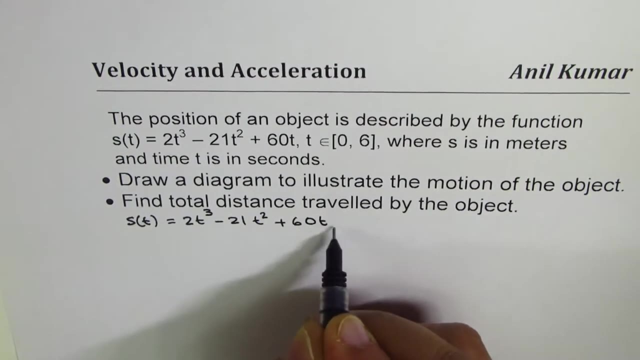 motion of the object. Find total distance traveled by the object. So let me rewrite all the above, the equations. First is displacement, which is 2t cube minus 21t square plus 60t. We are talking about t, which is belonging to the interval 0 to 6, correct. Then the derivative. 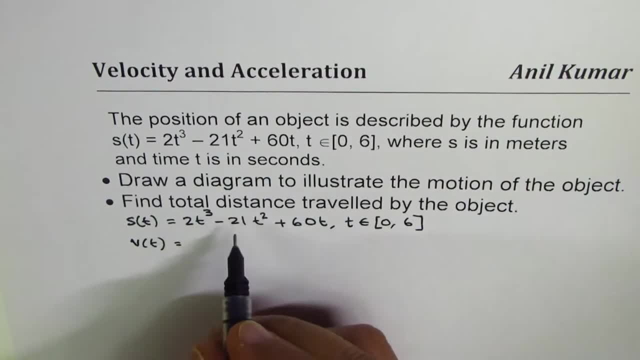 which is the velocity is. we got this as 6t square minus 42t plus 60.. And we also wrote this in the factored form after taking 6 common as t minus 2 times t minus 5, correct. 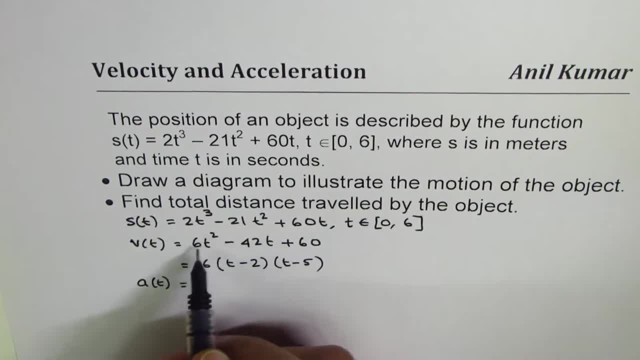 And then we found acceleration, which was derivative of this, which is 12t minus 42.. Now the first question which we need to address is draw a diagram to illustrate the motion of the object. So let us understand what kind of diagram to use. First, let us 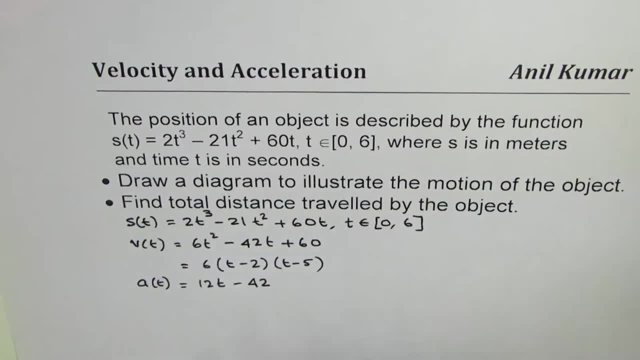 we need. So diagram we need is displacement with time, right, Let's say this is a linear motion along a straight path, right? So with that we'll make a diagram. So what we also see here is that there are two points. These are the turning points. We found that the velocity is 0 at t. 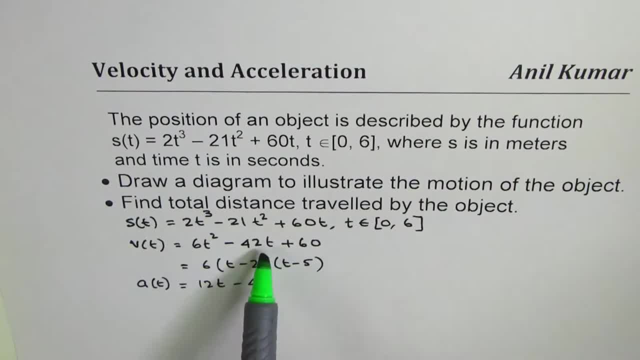 equals to 2 and at 5, correct. If t is 0, velocity is 60. So initially the object moves in the forward direction with initial velocity being 60. At t equals to 2, velocity is 0. That means it. 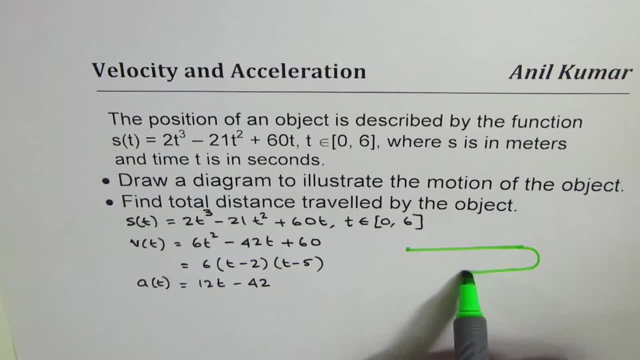 turns, That means it turns, correct, It turns, And when the time is 5 seconds it turns again. So it turns again, Kind of like this. right Now, relative positions we will find. So let's begin from the 0. At this. 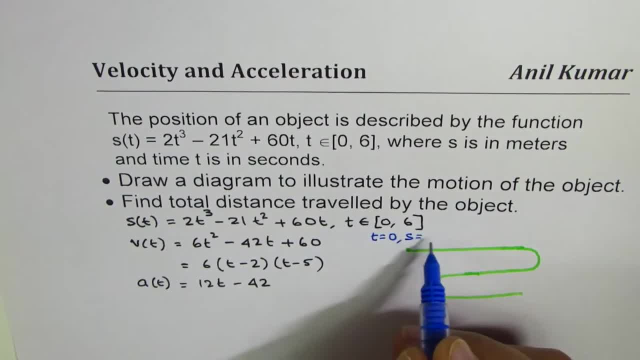 time t equals to 0. And what is the displacement or the position? So, at 0, s is also equal to 0, right, t is 0, s is 0. So we got it from the first equation. 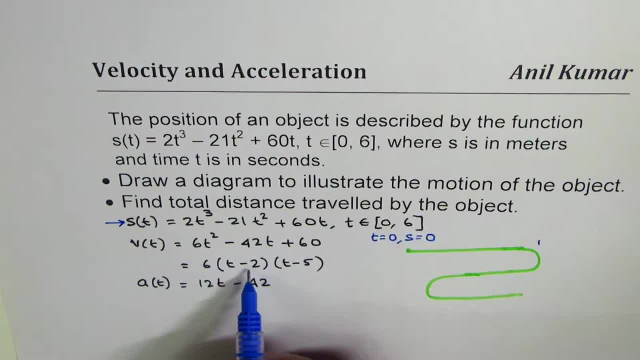 Here, at this position, it is a turning point when velocity is 0. So this is the time when t is equal to 2.. So if t is 2, what is s equals to right. So what we need to do is substitute 2 in this equation. 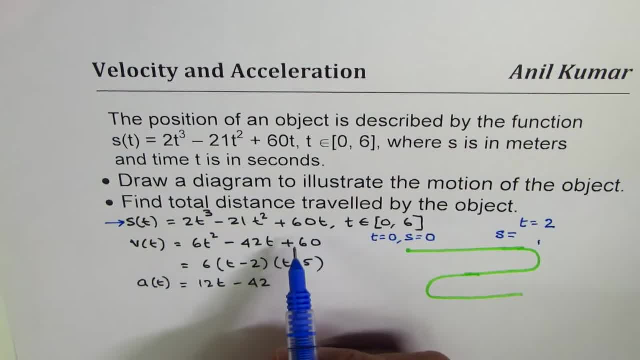 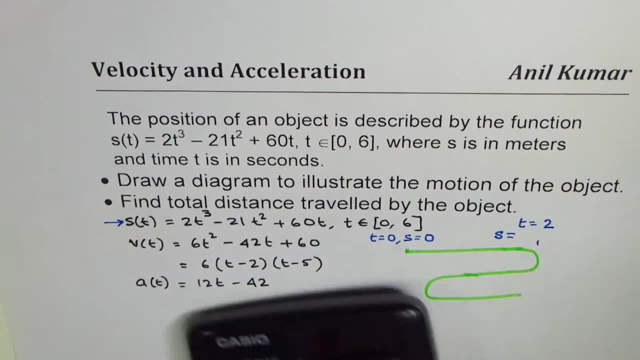 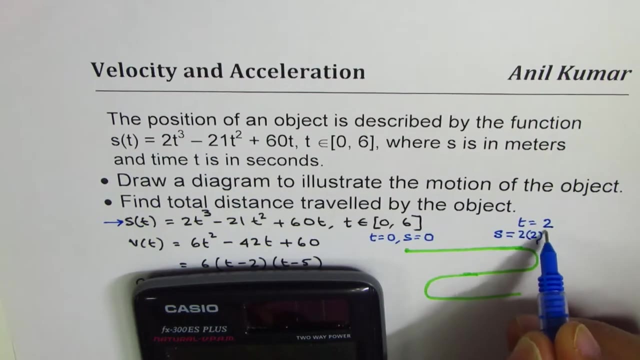 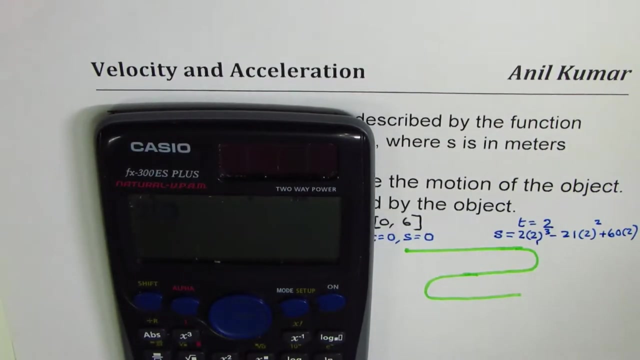 and then find the value of s. So let me get a calculator to do the calculations, right. So here we are. So we'll just substitute 2 in this equation. So we have 2 times 2q, 1 times 2 square, plus 60 times 2, right? So let's do it. We have 2 within brackets, 2q. 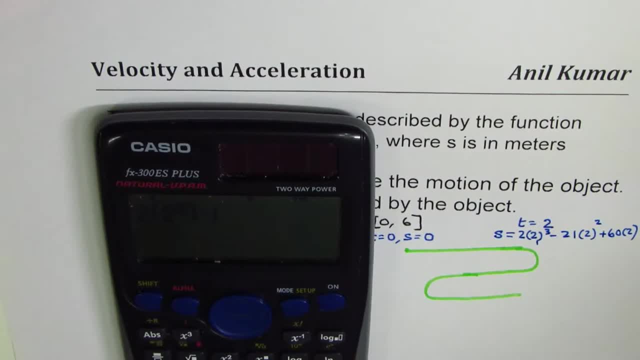 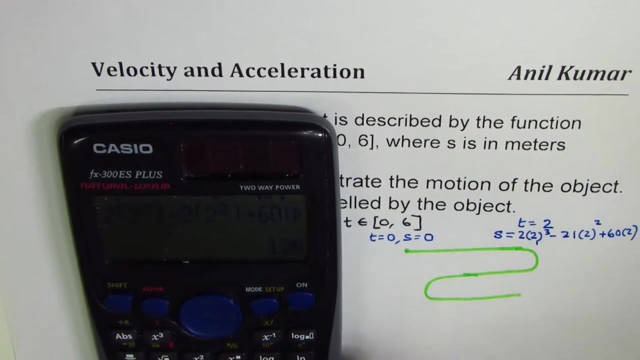 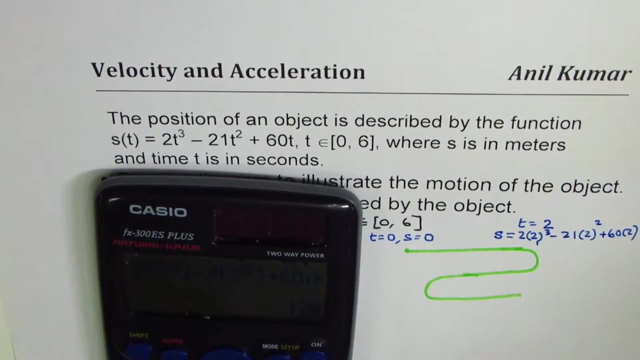 minus 2 times within brackets, 2 square plus 60 times 2. And that gives us 128.. So we get this distance. Sorry, this was 21 times, not this is 21. I wrote it wrong, So let's get. 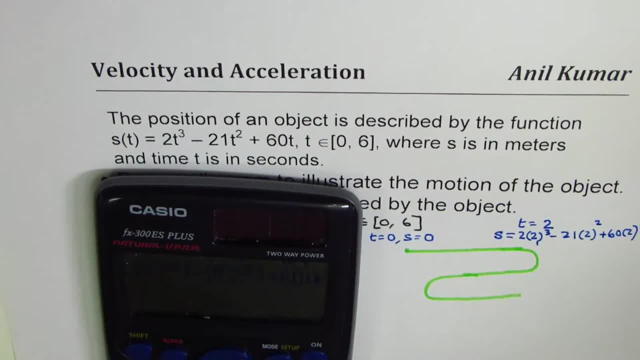 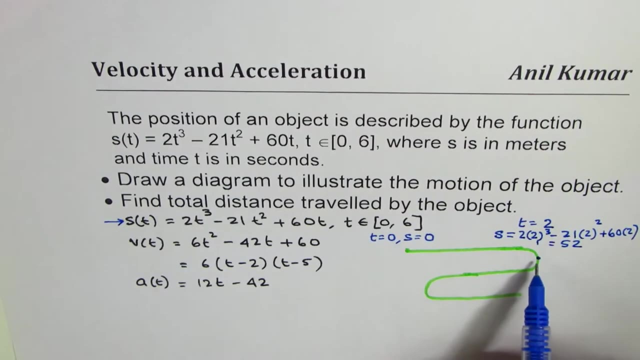 corrected, So it gives us 21 times 2, which is equal to 52.. So we get this position as 52, right? All units are in meters. So this happens at this point: At t equals to 2, the object returns and the displacement is 52.. Distance traveled is 52.. 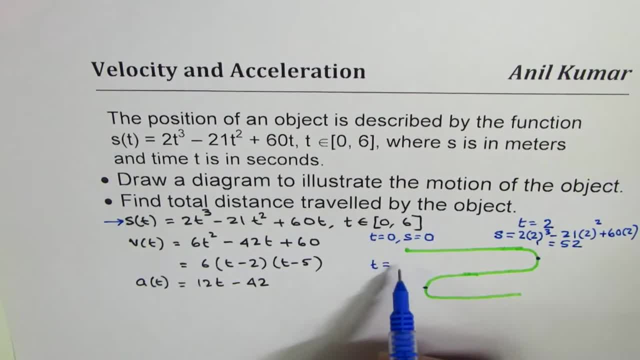 Now what happens at t equals to 5?? At t equals to 5, let's find what is s of 5.. So let me calculate here. So s of 5 is equals to 2 times 5q minus 21 times 5 square plus 60 times. 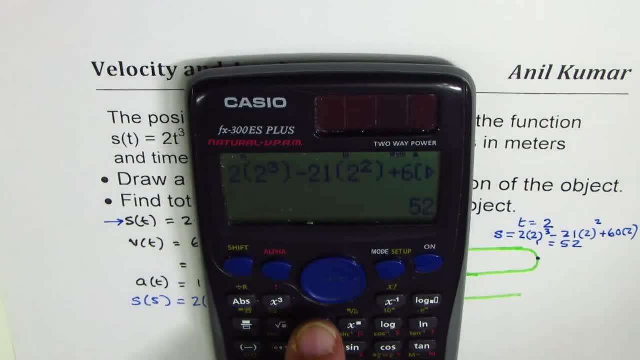 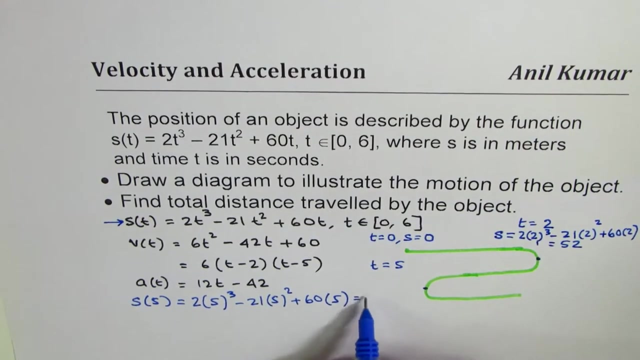 5, correct. So in this equation I will change 2 to 5.. So that gives us 5 here, 21 times 5 square and 60 times 5, which is equals to 25.. So we get this as 25.. So s at this position is 25.. Is it okay? 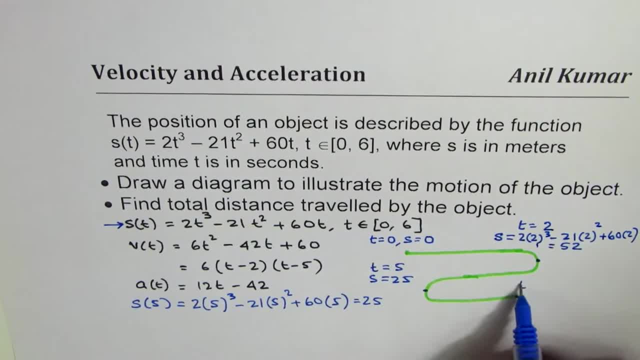 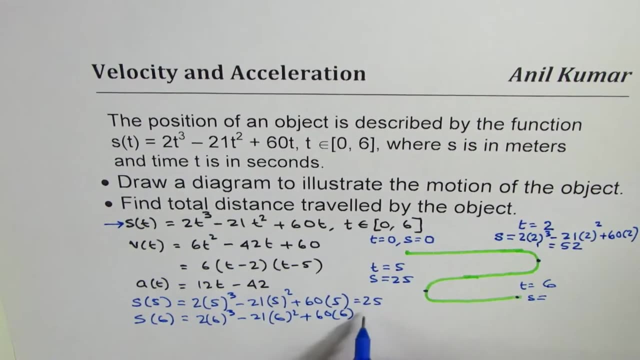 Let's also calculate at the end: when t equals to 6, right, Then s is equals to. so at 6, s is equals to 2, 6q minus 21,. 6 square 60 times 6 equals to how much? So we'll change 5 to 6 now. 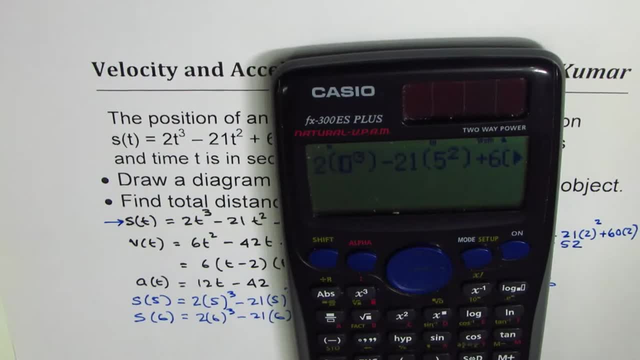 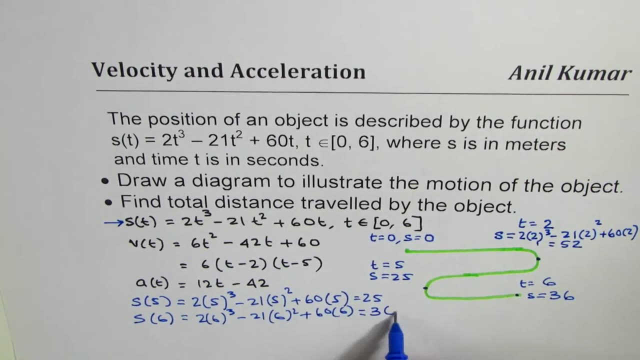 6.. 21 times 6 square and 60 times 6. That gives us 36.. 36, right. So that is the displacement with time graph. The object starts at 0 position, Displacement is 0.. It returns after traveling. 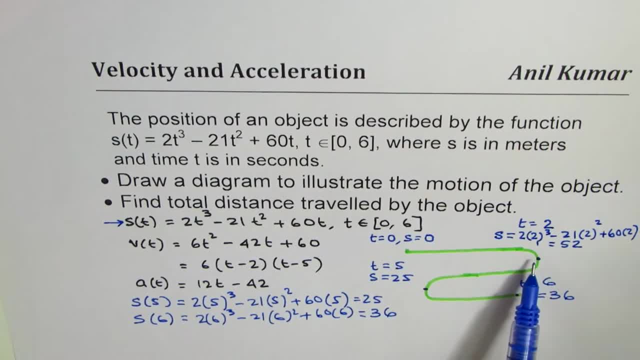 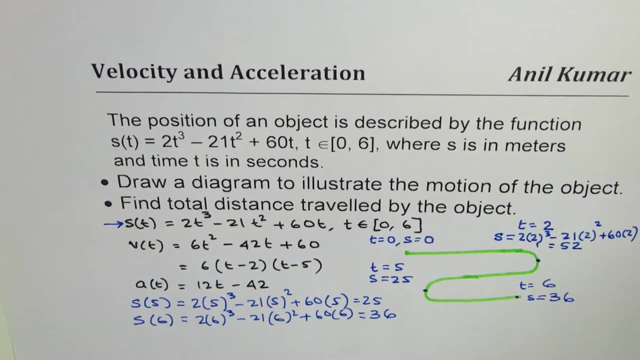 a distance of 52 meters and then travels backwards, It reaches the position 25.. After 5 seconds, that is, and the last second, it travels further in the positive direction, correct? So that becomes the diagram. Let us calculate the total distance traveled by the. 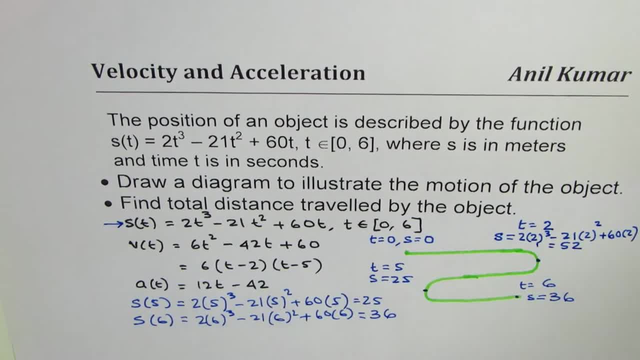 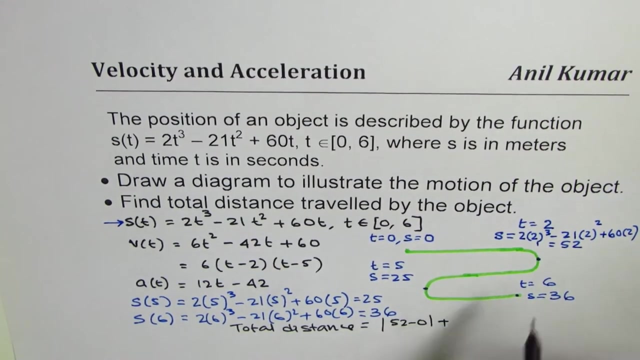 object. So the total distance is. let's calculate sum of all these distances traveled, right? So in the first lab, while moving forward, distance is 52 minus 0.. Now we are calculating total distance. Distance is always positive, right? So it is positive value of 52 minus 0 plus. then we have